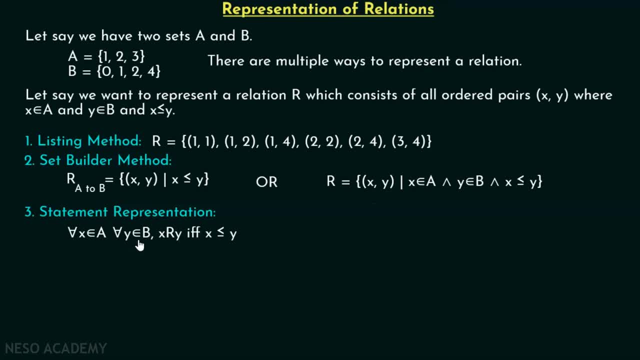 okay, For all x belong to A and for all y belong to B. x is related to y if, and only if, x is less than or equal to y. Simple, right Now. the fourth representation that I want to discuss is matrix representation. This is quite simple representation and sometimes it helps us in finding the solution. 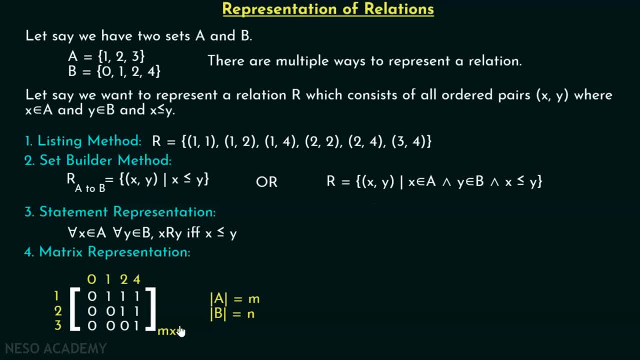 of the questions easily. okay, This is how we can represent representation R Here. let us suppose the cardinality of A is m and cardinality of B is n. That means we have m elements in set A and n elements in set B. Then obviously we can easily. 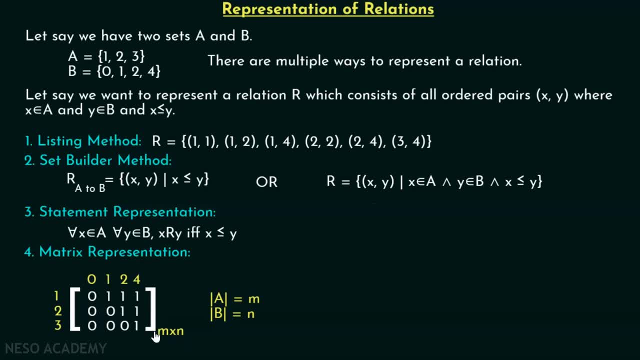 create a matrix of size m cross n right. There must be m rows and n columns in this matrix right. Here in this example, obviously we have three elements in set A. Therefore three rows must be there in this matrix and we have four elements in set B. Therefore, 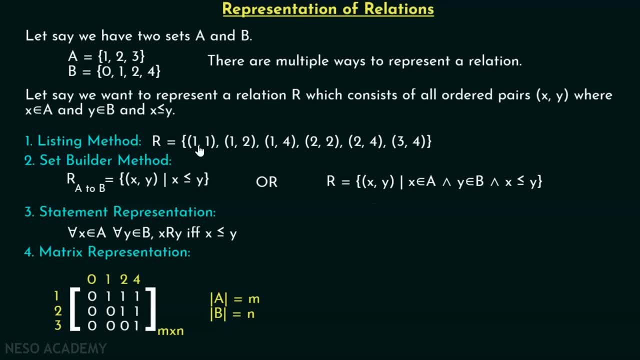 columns must be there in this matrix And in order to represent this ordered pair 1, 1, we must put 1 in this particular position, that is, in this cell. This cell represents the ordered pair 1, 1.. Putting 1 over here means that we are including 1, 1 in relation R. Similarly, 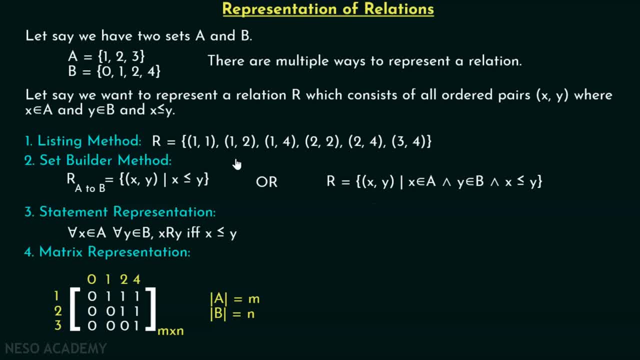 putting 1 over here means that we are including 1, 2 in relation R, right, And you can see over here that 1, 4 is also included in R. Therefore, we must put 1 over here, as this cell represents. 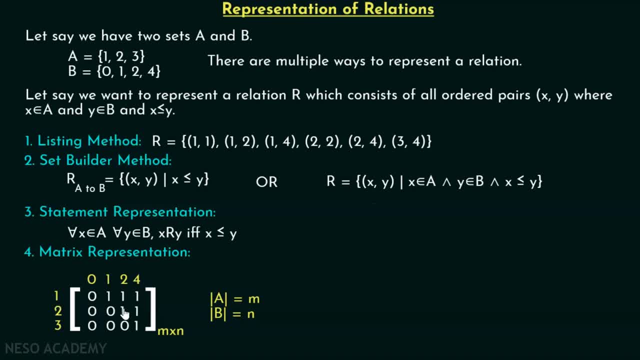 the ordered pair 1, 4, right. Similarly, we can put 1 over here and 1 over here. Also, we can put 1 over here. This cell represents ordered pair 2, 2.. This cell represents this. 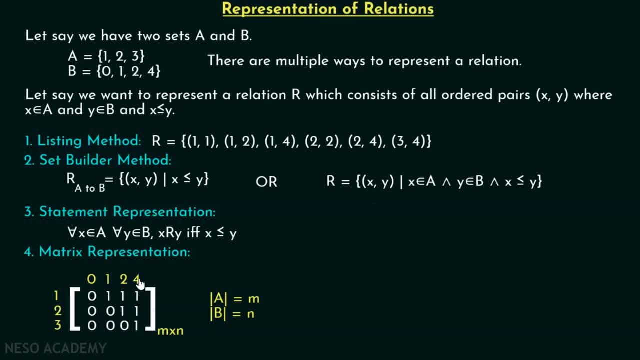 ordered pair 2, 4, and this cell represents this ordered pair 3, 4, right. So this is the matrix representation of relation R. Now the fifth representation is graph representation. okay, And that too, we are considering directed graph. Here, you can see I am representing all the 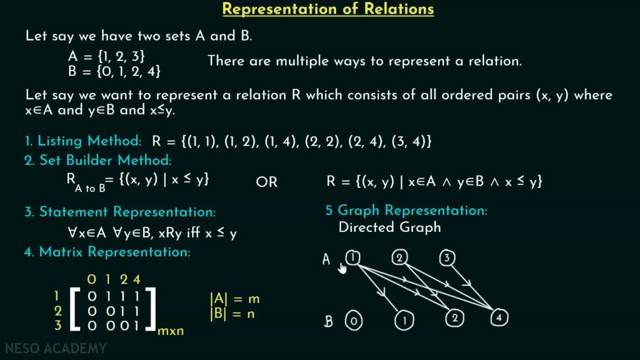 elements of set A and set B by these nodes. right Here I have written all the elements of set A and here I have written all the elements of set B. These nodes are representing the elements of set A and these nodes are representing the elements of set B. okay, And here you can see I have drawn